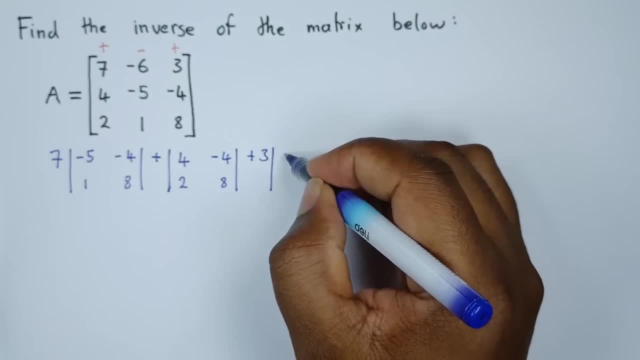 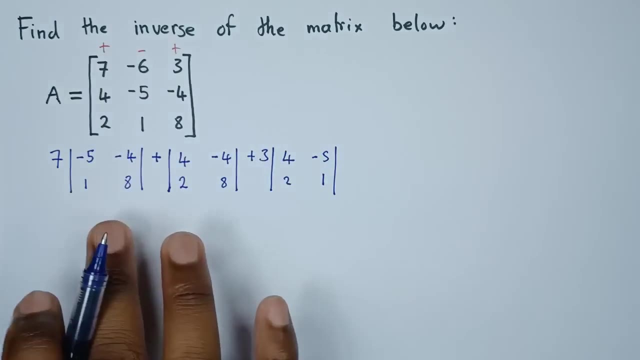 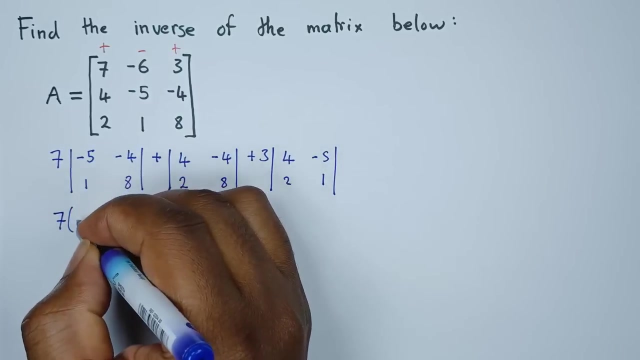 last value that we have, there is a three. What's the two by two formed? Same concept: Four. two negative five, one. Okay, So now let's find the determinants of this particular two by two that we have. So we're going to say seven Negative five times. eight is negative forty One times. 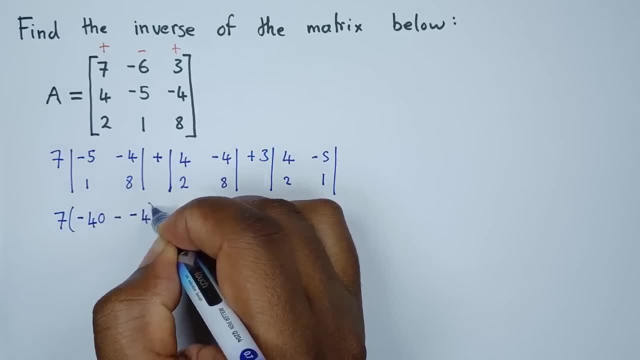 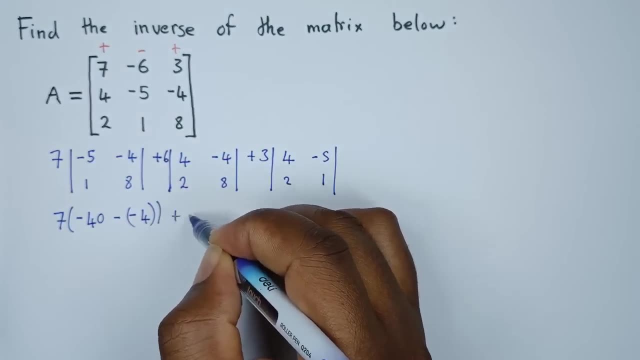 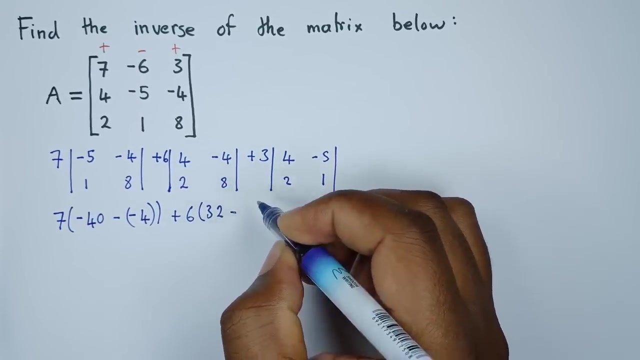 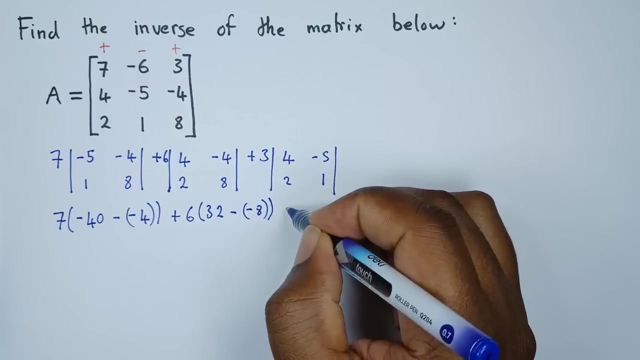 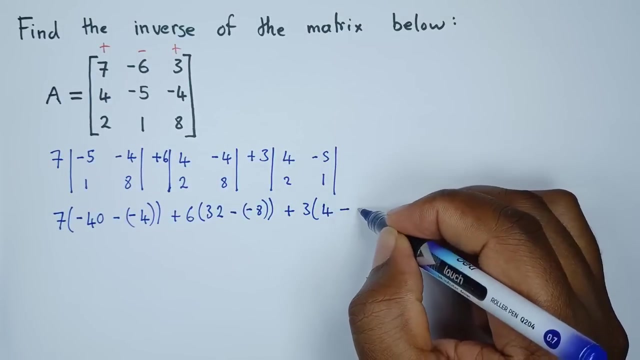 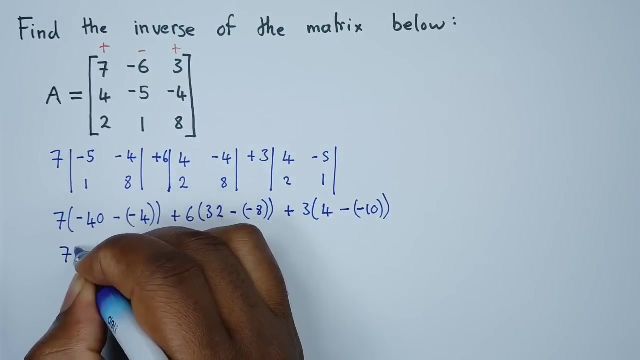 negative four is negative four Plus. so we left out a six here. So plus six, Then four times eight, we simply get 32.. Minus eight times, sorry, two times negative four is negative eight Plus three. Four times one is four. Minus two times negative five is negative ten, Like that. Okay, So let's see how it proceeds. So here we have seven multiplied with So forty, and negative, negative four, Simply get. 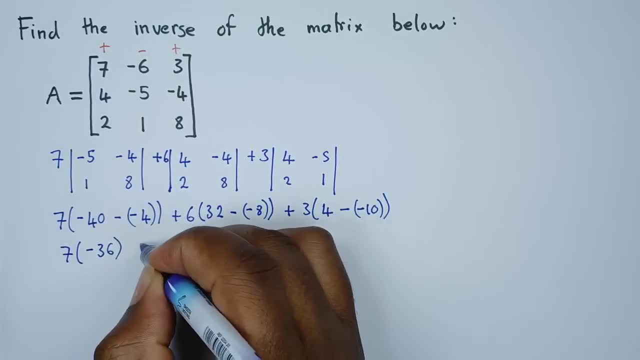 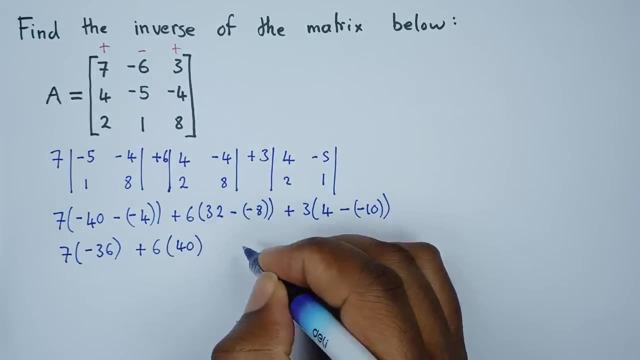 negative thirty six, Then plus six, Here we have 40.. Like that. Then, lastly, there we have plus three. In the brackets we'll get a 14. Like that. So now let's just expand and then add everything. we see what we get as our. 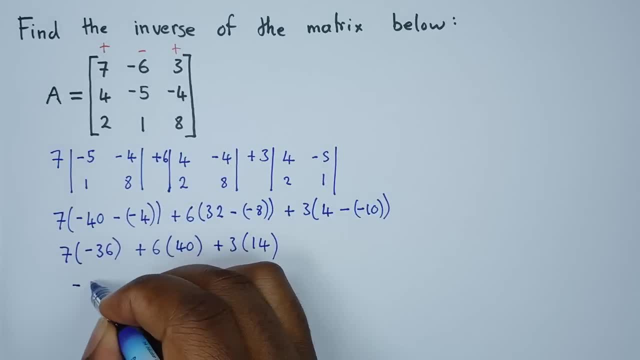 determine and best. So thirty six multiplied by seven, we seem to get a negative 252.. So, plus so, 40 by 6, you get a positive 240. and lastly, 14 multiplied by 3, you get a positive 42, like that. so if we add all these values together, what we're going to get will be positive. 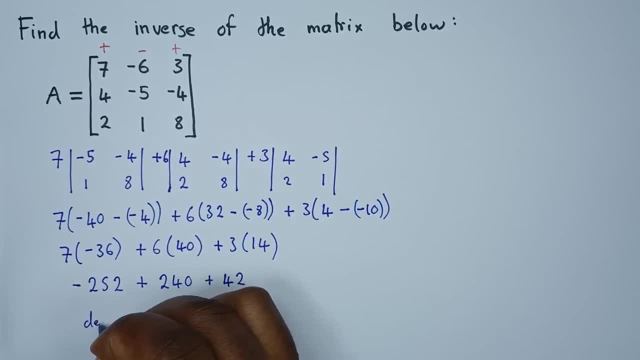 30. so the determinant of this matrix a is equal to 30.. so this is the first step. step number one: find the determinant of the particular matrix of which we've done. the next step now is to find the cofactors. so let's go ahead and find. 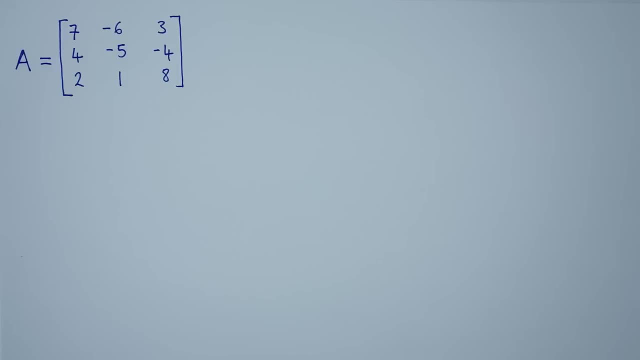 the cofactors. okay, so we're back to our matrix a. so to find the cofactors, we're going to be picking each particular digit in this case, and creating a two by two matrix. so, for example, if we pick the first value, which is a seven, we're going to hide the row for seven. 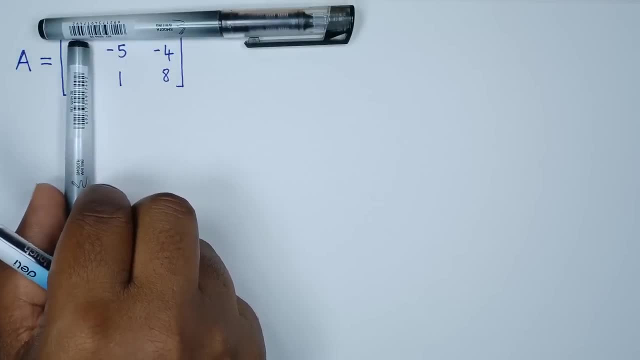 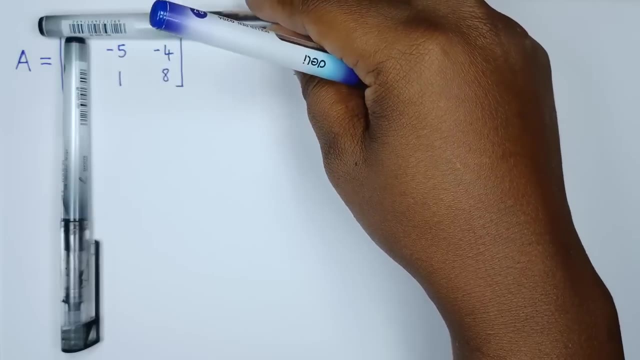 as well as the column for seven. so whatever remains creates the two by two that we're looking for, just like that. another example is, for example, if you pick a four, that is here, we're going to hide the row for four as well as the column for four, like that. then whatever values are remaining, 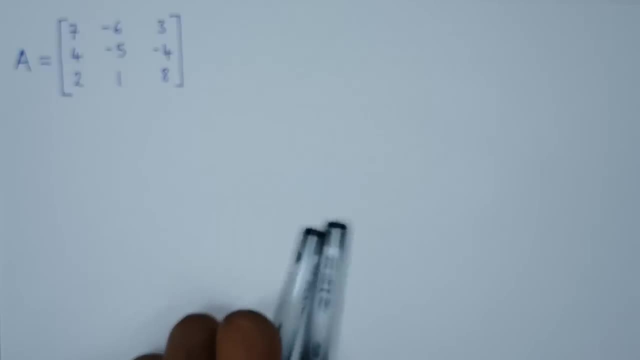 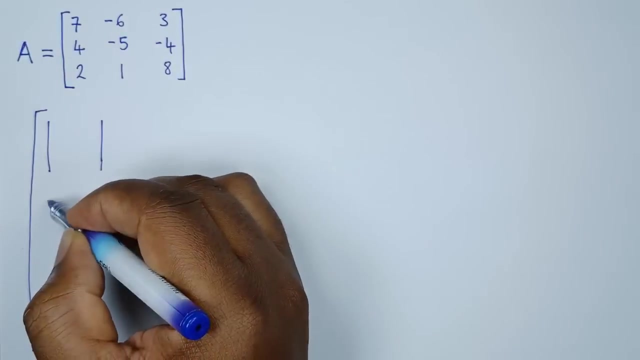 will create our two by two matrix that we're looking for. so, to do that, we're going to have a very big matrix. so it's a very big matrix, yeah, something like this. so let's create our two by two matrices and this is what will give us our cofactors. so we have this. 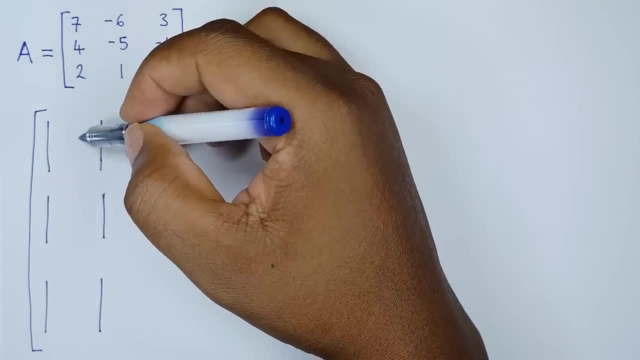 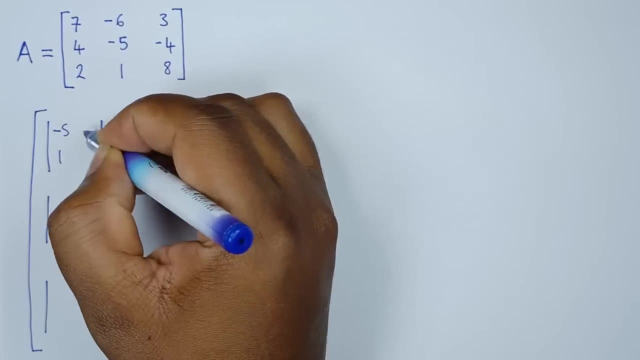 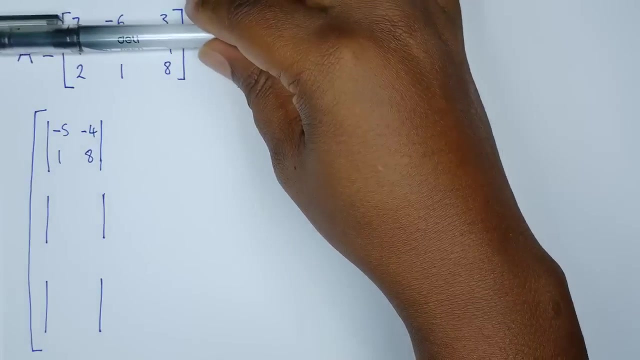 so at this position, of course there's a seven there. so at this position, if we put uh, if we exclude the row and column for seven, the two by two formed will be negative five, one, negative four and eight, like that. if we move on to the next number, which is uh, four, if we hide the row as well as the column for four, 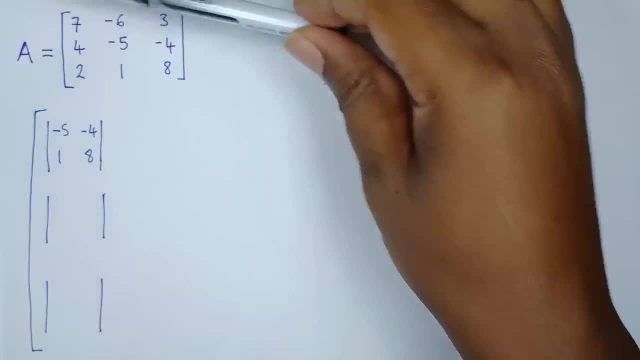 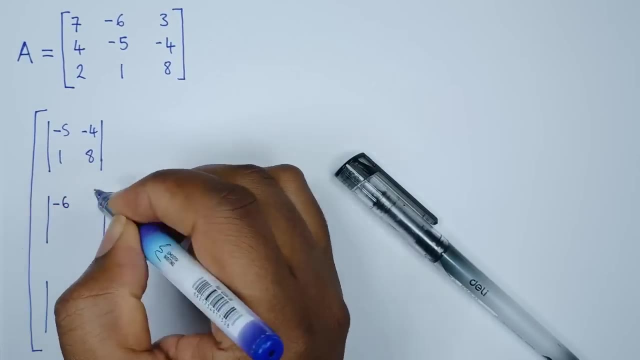 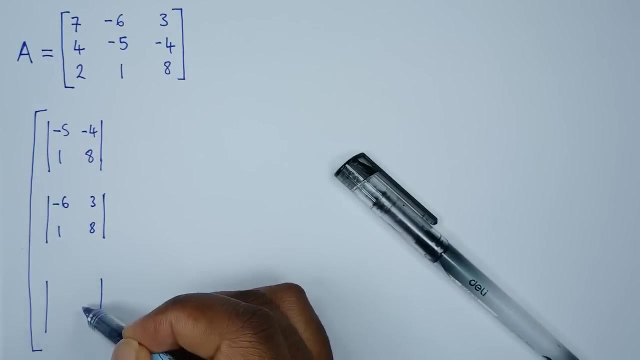 the remaining values is what uh gives us, the two by two we're looking for. so the remaining values, of course, will be: we use the same color. the remaining values will be negative. six here, three, one, eight, like that. i hope you get the concept. now, same thing, uh, for this particular matrix here. 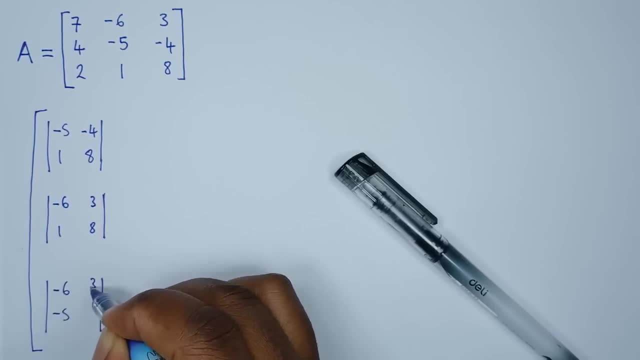 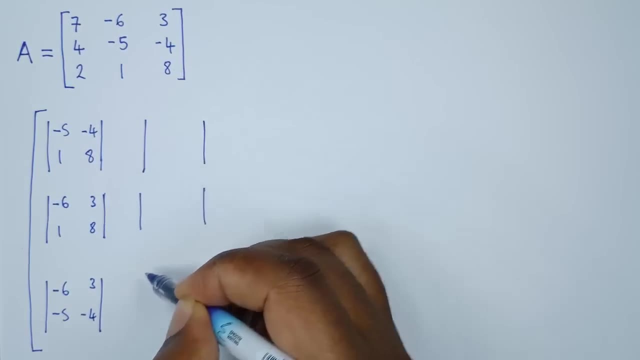 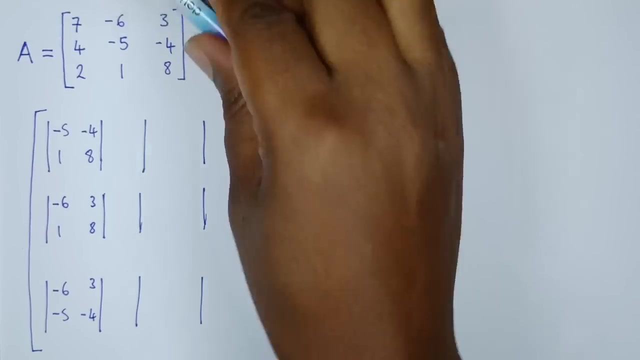 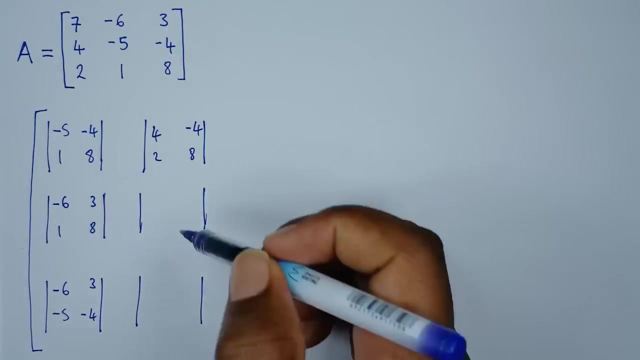 we'll have negative six, negative five, three and negative four. okay, so let's move on to the second column. so this is our second column, so the second column. what will be formed here? everything excluding this row and this column. so we have four, two. here. we have negative four. here we have eight. the next one is at five there. 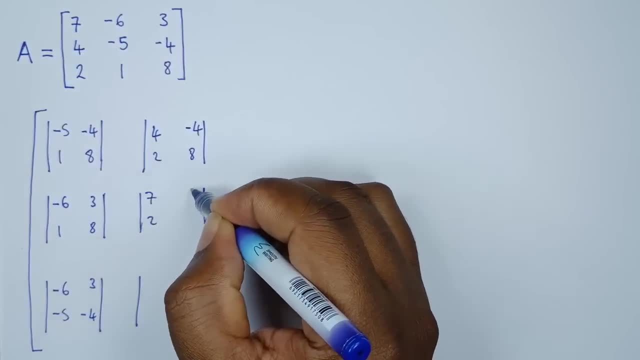 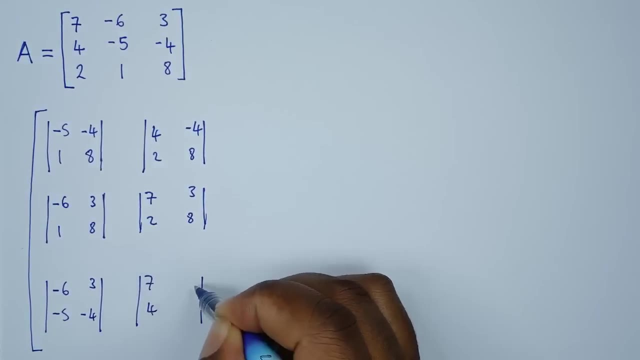 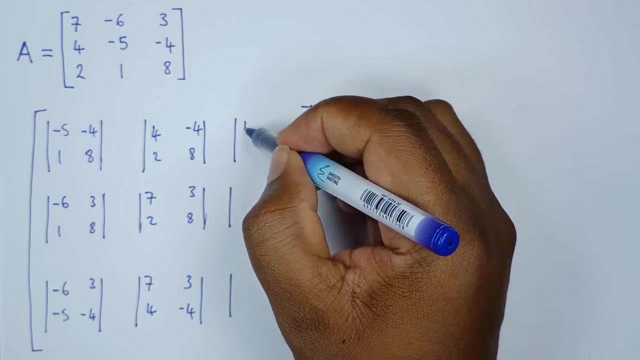 so, excluding the row and column, we'll have seven, two, three, eight. the next one is one row and column excluded. So 7, 4, 3, negative 4.. Let's include the last column like this: Okay, So the 2 by 2 that will be formed here will be 4, 2, negative 5, 1.. 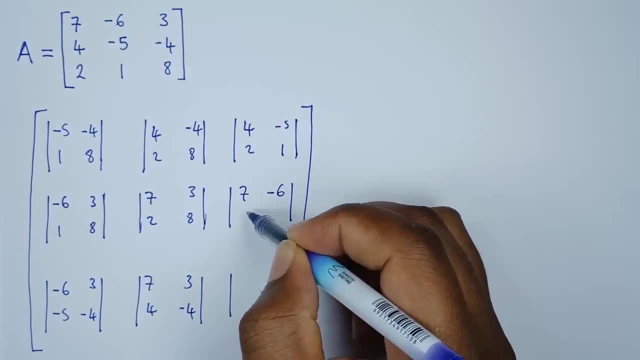 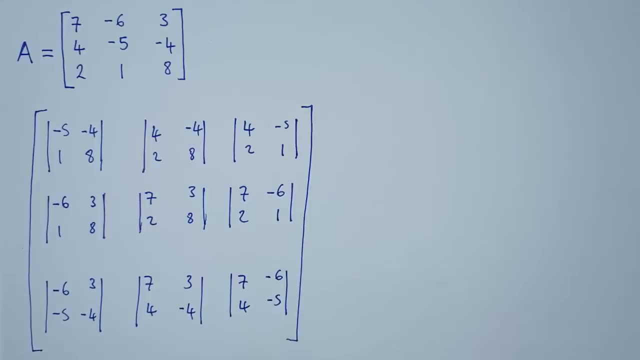 At this position, the 2 by 2 formed will be 7, negative 6, 2, 1.. At this position, we have 7, 4, negative 6, and negative 5.. Okay, So we have filled up everything and this is what we have. 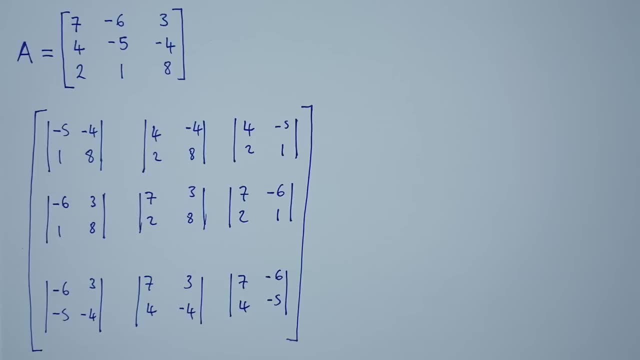 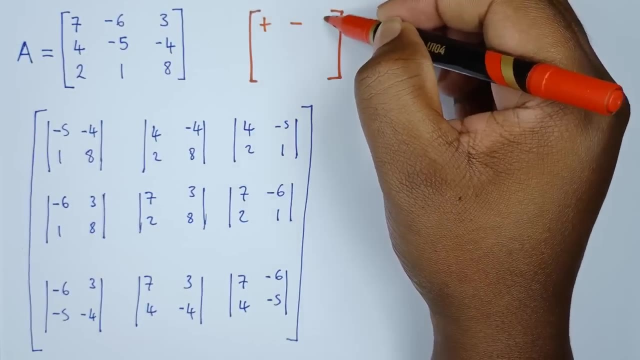 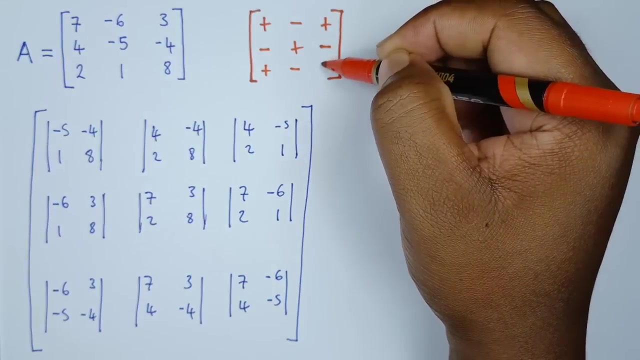 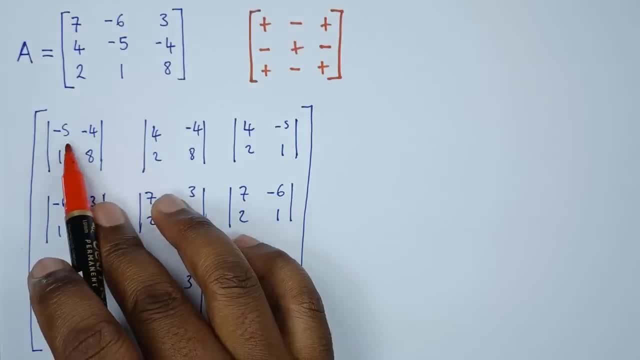 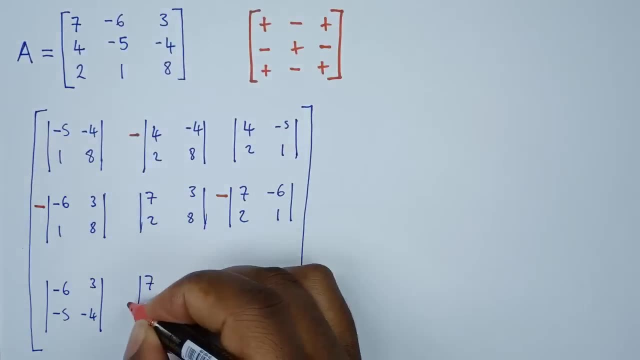 Okay, So, based on these positions, this matrix will be positive. this matrix here should be negative. So this one here negative, This one here negative, This one negative And this one negative as well. So whatever determinant we're going to find at this position, we're going to include the negative part as well. 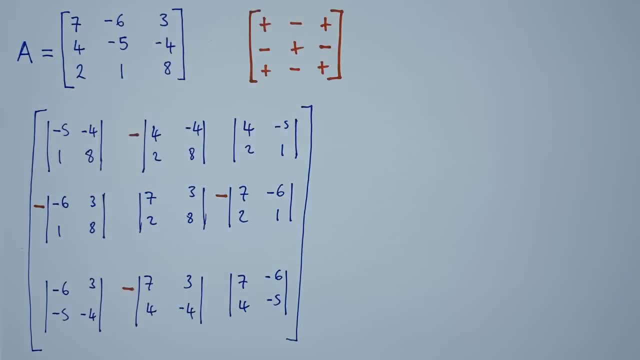 Then if it is affected, it will obviously change. So now the next step will be to find the determinant at each position. We're finding the determinant at each position And this is what we're going to get, So let's go into that. 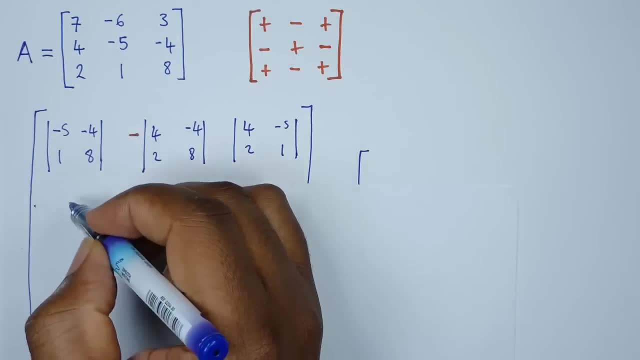 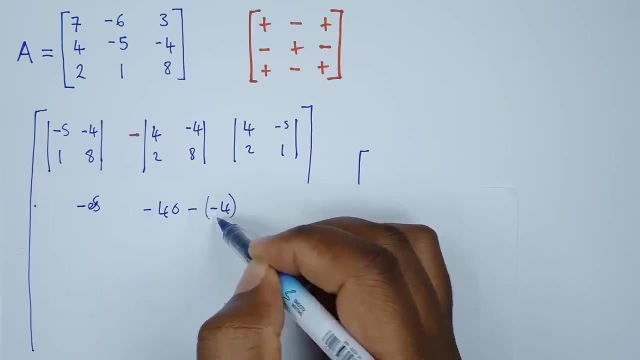 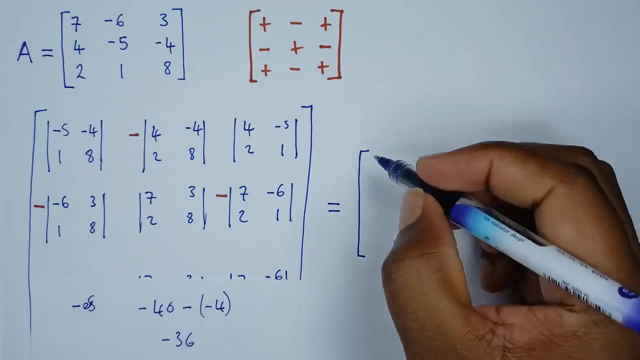 So the first matrix that we have, Which is this one: here We can say negative 5 by 8. Let's just say negative 40 minus negative 4.. So the determinant there will simply be negative 36.. So we write our negative 36 right here. 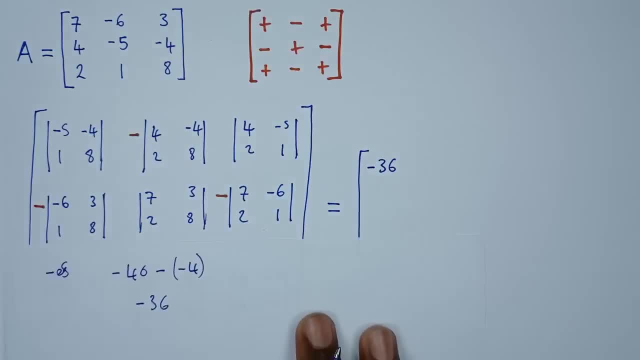 Negative 36.. Move on to this matrix here In which we're going to say: 4 times 8 is 32 minus negative 8. Like that, So we're going to get a positive 40. Now remember there's a negative outside. 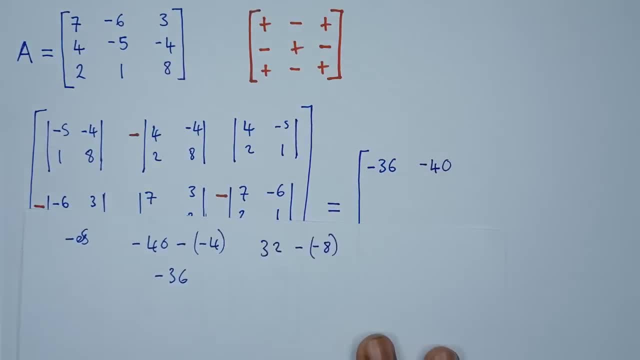 It has to become a negative 40 instead, Like that. And the last one is 4 times 1,, which is a 4. Then 2 times negative 1. So negative 5 is negative 10.. Like that. 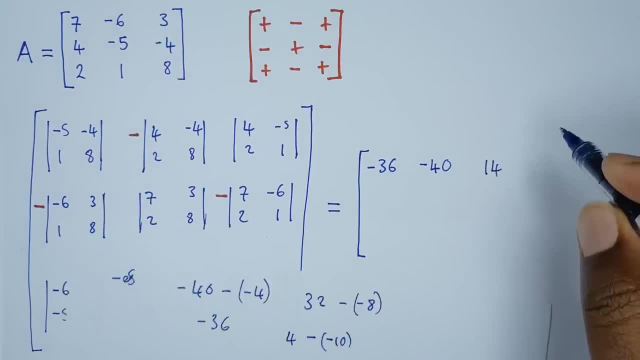 If we add the 2, it's going to get 14.. So that's basically the idea. So the next thing now we're going to do is find the determinant at each position. So let's go ahead At this position here we'll have negative 6.. 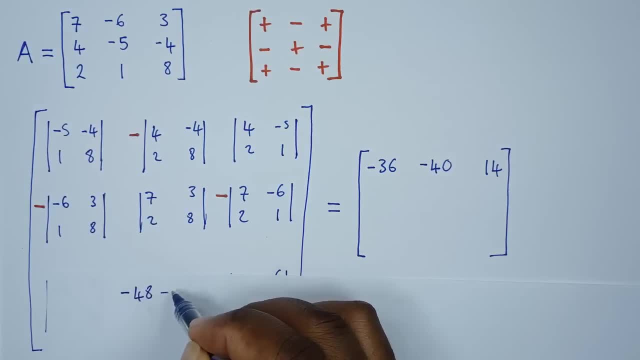 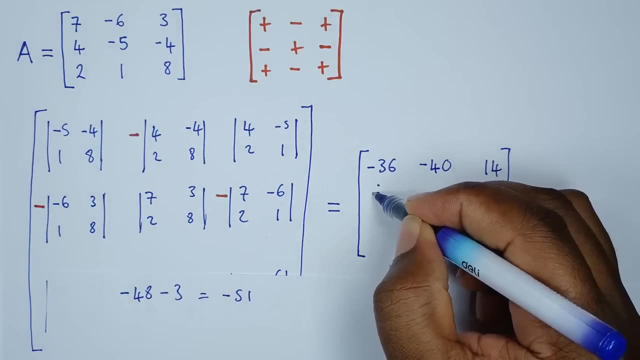 So 6 times 8. That is negative 4H minus 3. So this should give us negative 51.. Now remember there's a negative outside, Hence we get a positive. So in here positive 51.. 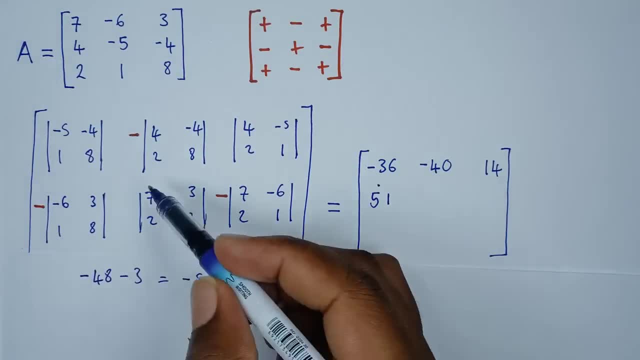 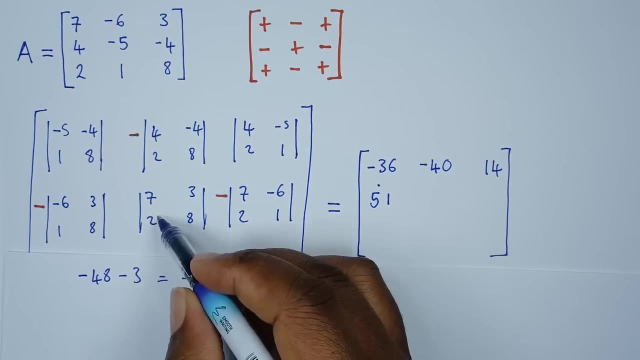 Let's find the determinant here: 7 times 8. That should be 56.. So 56 minus 6.. The product of these two, Hence, we get 50. So here we have a 50. We come to this matrix here. 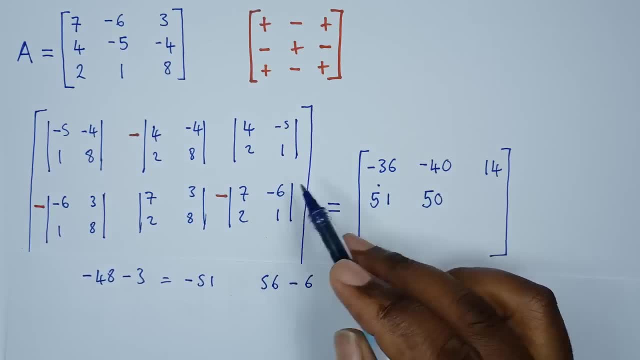 7 times 1. That is a 7.. 2 times negative 6.. So that is negative, 12. In brackets. So what we get here will be 19 positive, But remember there's a negative outside. 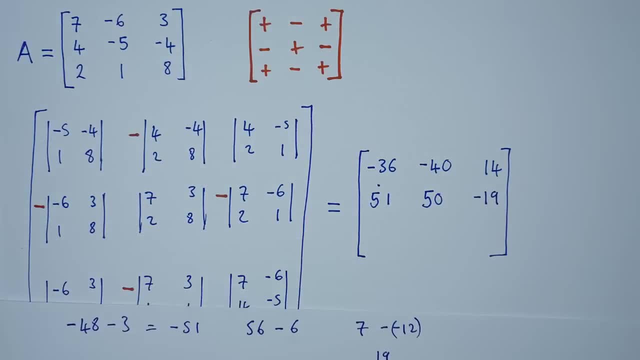 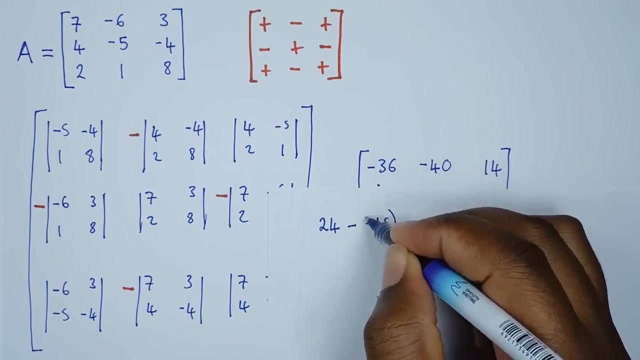 Hence, that is negative 19. Like that. The next step is this one here, So we can also say 6 times 4. Negative, negative, That is positive 24.. Minus Minus negative, 15. Like that. 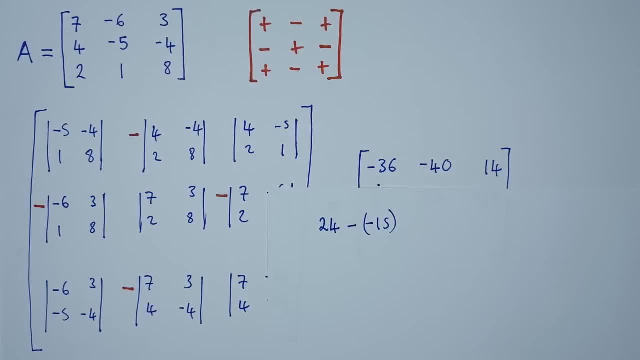 So again, just similar to what we've been doing. We just put them together And what we get will be a positive 39. So here we have positive 39. We come to this matrix here. 7 times 4 should be negative 28.. 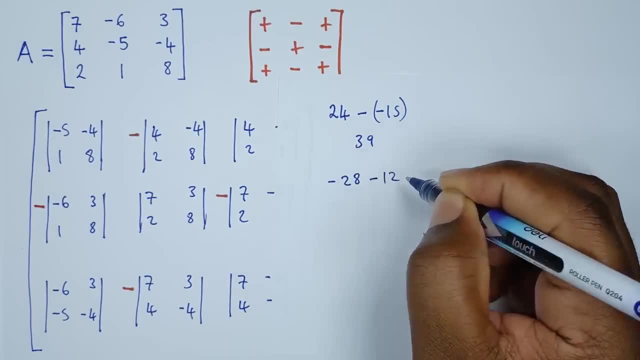 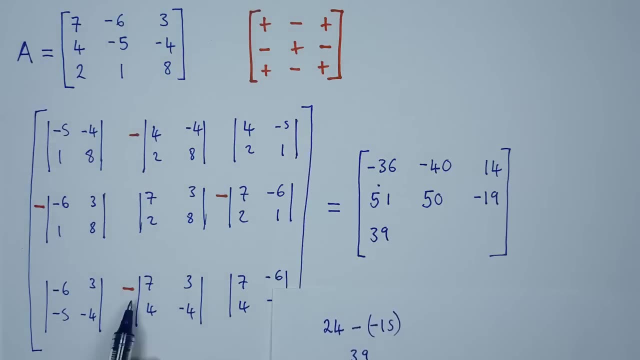 So negative 28 minus 12.. So this should give us a negative 14., If I'm not mistaken. Now, remember, there's a negative outside, Hence this will become positive. Positive 40.. The last part, which is this one here: 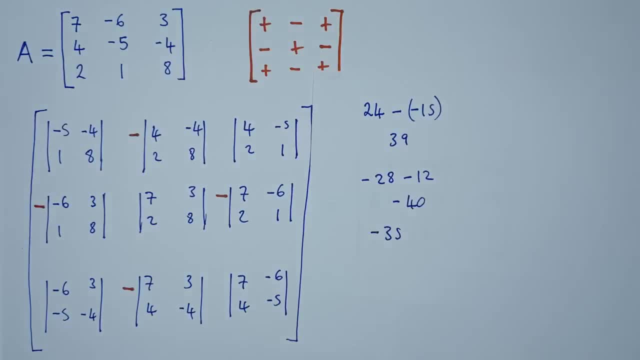 7 times 5 is negative 85. Then 4 times 6 is negative 24.. Like that, So this becomes negative 35 plus 24.. So subtracting the two, we should get 6 plus that. 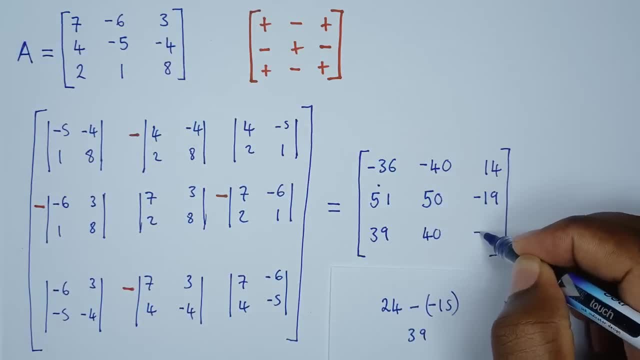 We get a negative 11.. So this here is negative 11. Like that. So So, after finding all these values- these are the cofactors that we're finding- After finding all these values, what we're going to do is this matrix that we have here. 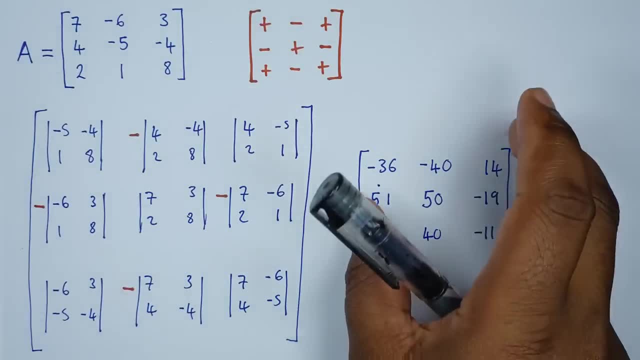 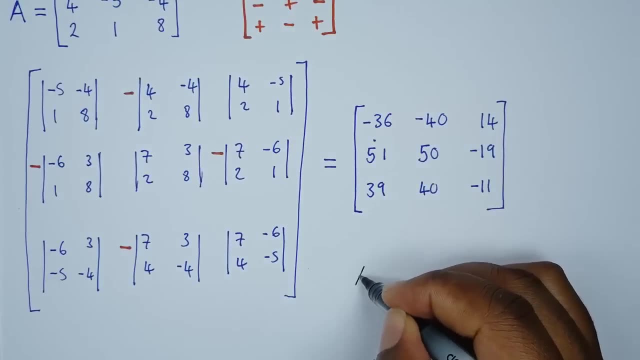 we're going to transpose it. Transposing this matrix that we have will give us the adjoint. So the adjoint of matrix A will be equal to the transposed cofactors. So let's transpose it. So the row becomes the column. 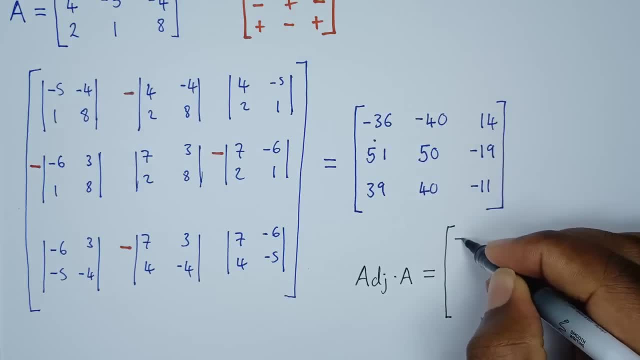 The column becomes the row. So the first row is negative 36, negative 40,, 14.. That will become the first column. The second row, 51, 50, negative 19.. The third row, 89, 40,- negative 11.. 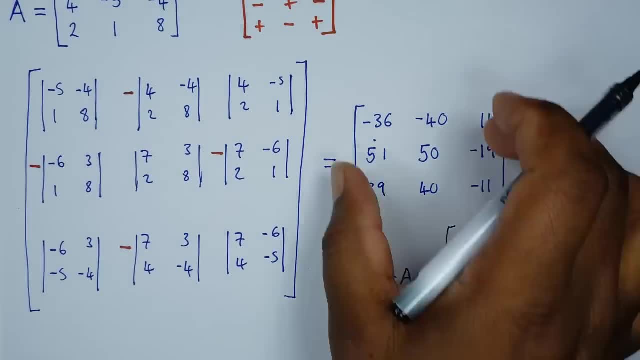 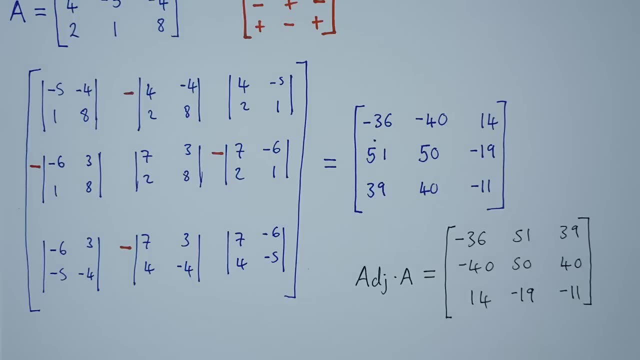 So this is what we have. So once we transpose this, what we get is a, The adjoint of A. Now remember: so far we have the determinant and the adjoint of A. Combining these two using the formula, we get our desired answer. 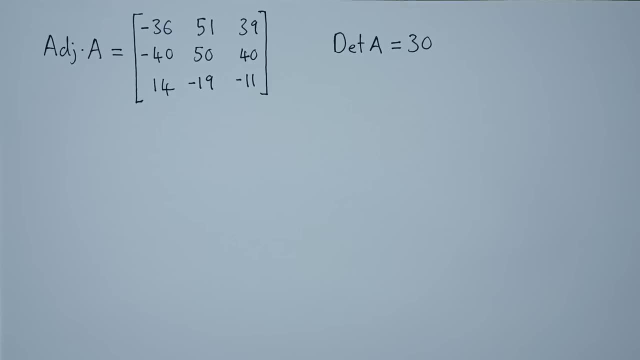 And that is the inverse. So let's combine the two. Okay, So from the beginning of the video, we had to find the determinant first, And the determinant we found to be 30. And this is our adjoint, after going through all the cofactors process. 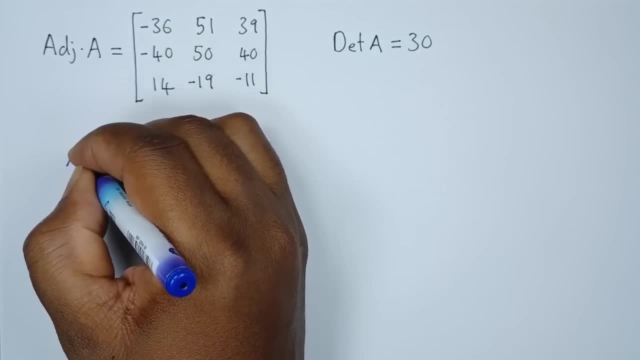 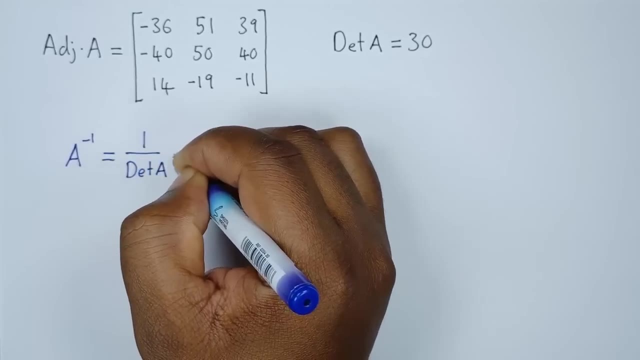 So now the formula for the inverse is given by inverse of A is equal to 1 over the determinant. So this is our adjoint of A multiplied by the adjoint of A. So this is what we have. Let's do this here. 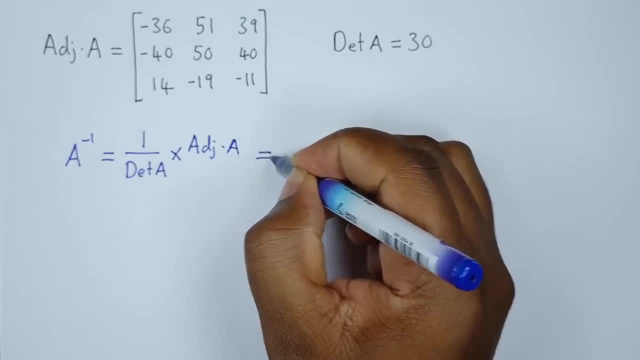 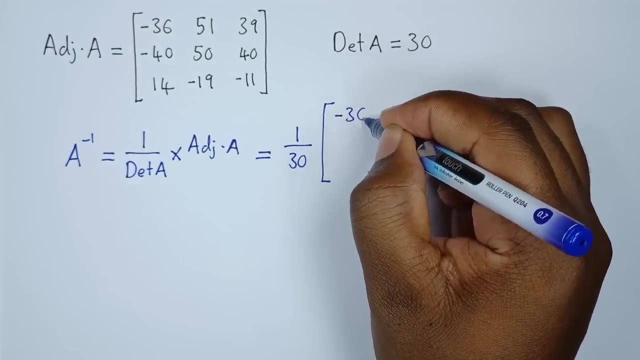 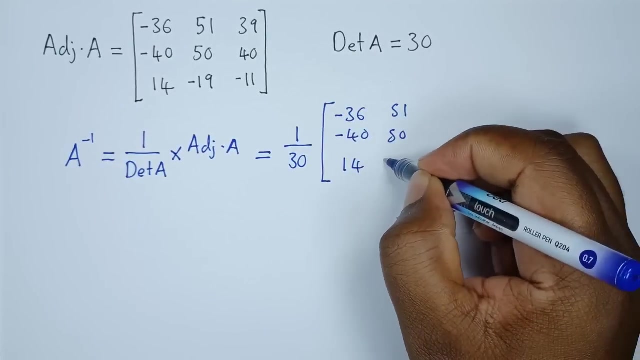 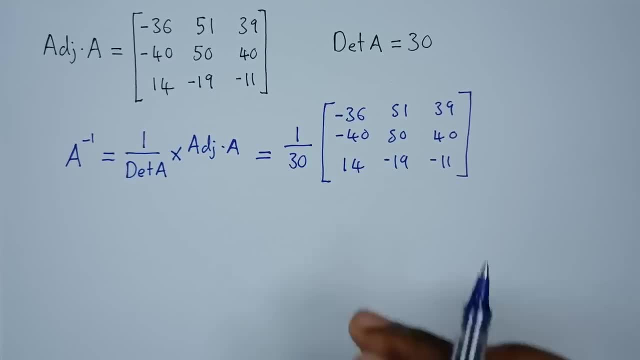 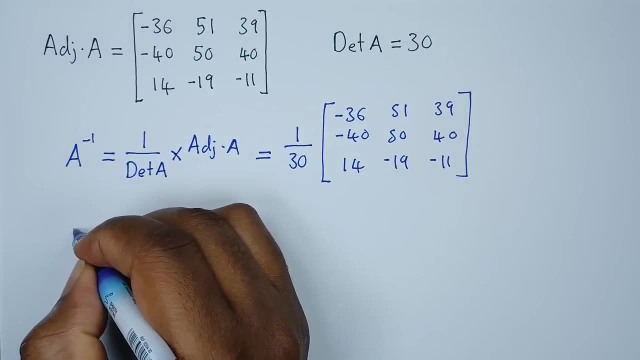 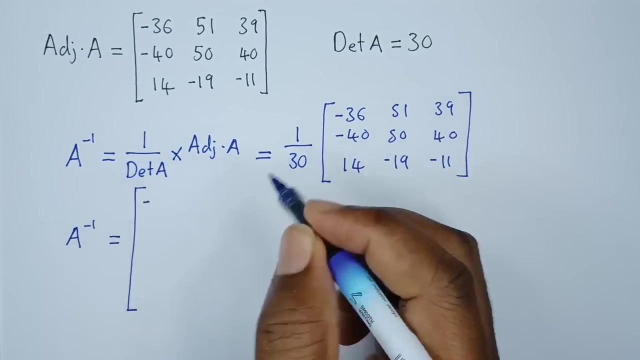 That's what we have, Okay, So now we are multiplying 1 over 30 times everything in this matrix and we can reduce where we can, where we have to reduce, So A inverse will be equals to: so we'll have negative 36 over 30.. 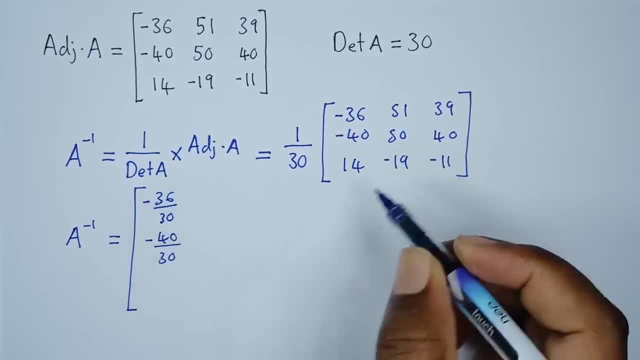 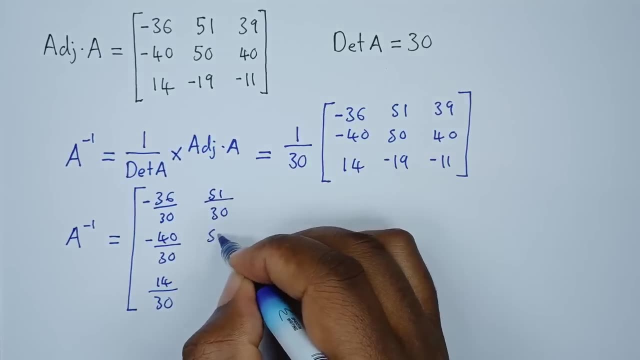 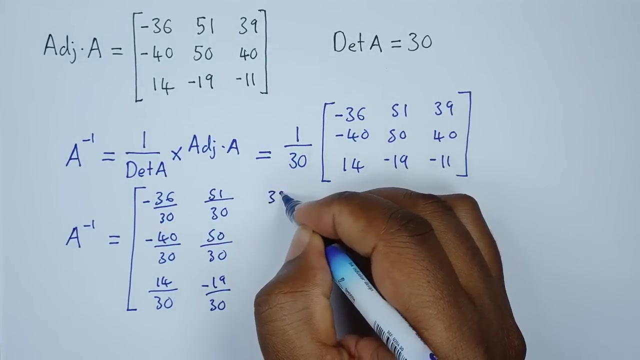 Next thing will be negative: 40 over 30. And lastly, we'll have 14 over 30, 51 over 30, 50 over 30 and negative 19 over 30.. last part: there we have 39 over 30, 40 over. 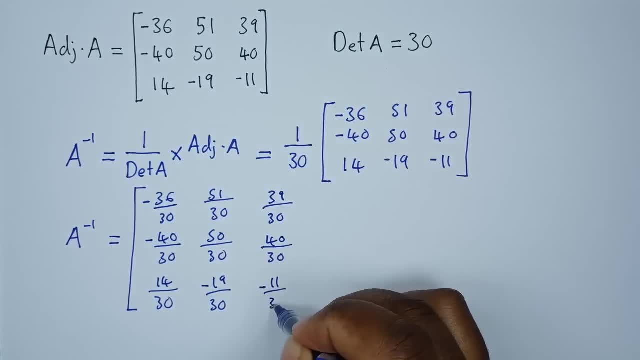 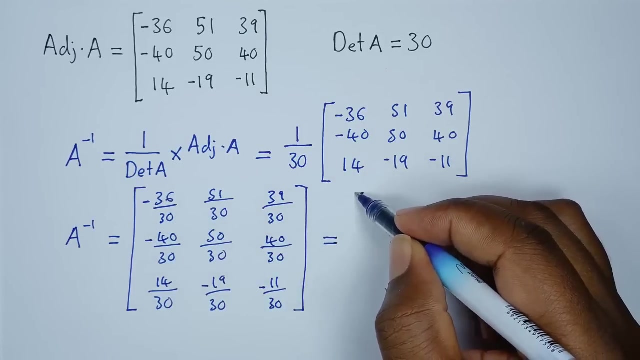 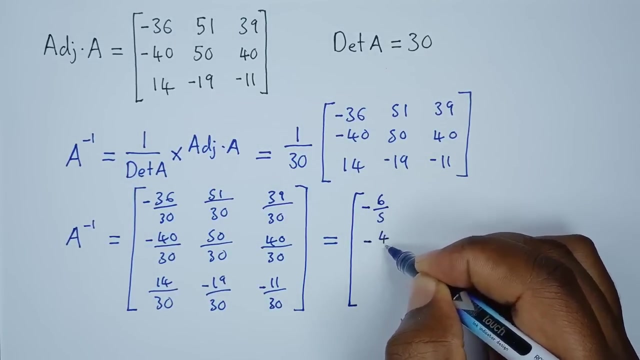 80 negative, 11 over 30, like that. so with this now we can reduce where we, where we, where we can. so for example, here we know that 6 can go into 36 and um and 30. so our final answer will look like this: 6 into 36 is 6, 6 into 30 is 5, so 6 over 5.. 10 into 40 is 4 into 30 is 3, so negative, 4 over 3.. 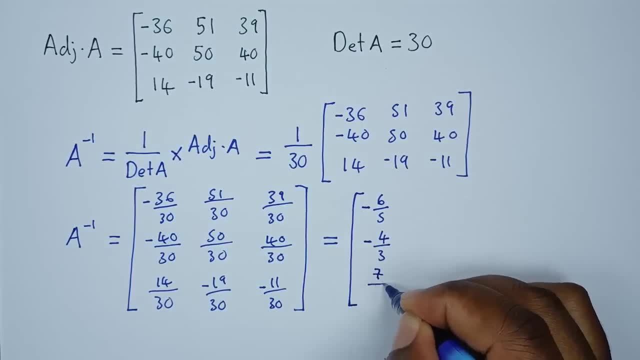 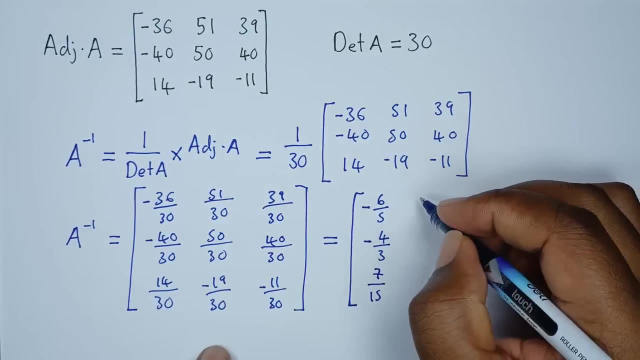 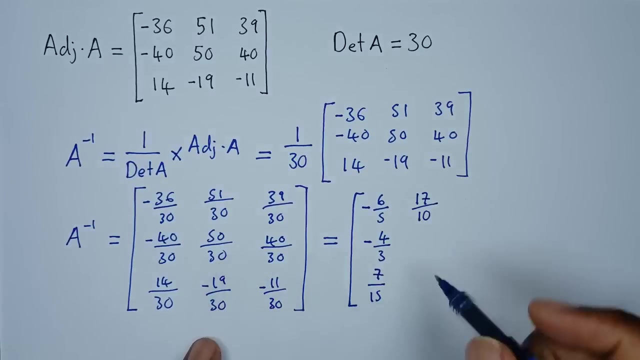 here 2, that would be 7 over 15.. here we have a 51 and we have 30. so 3 into 51, we have 17.. 3 into 30, we have 10.. and we come here and just cancel the zeros. 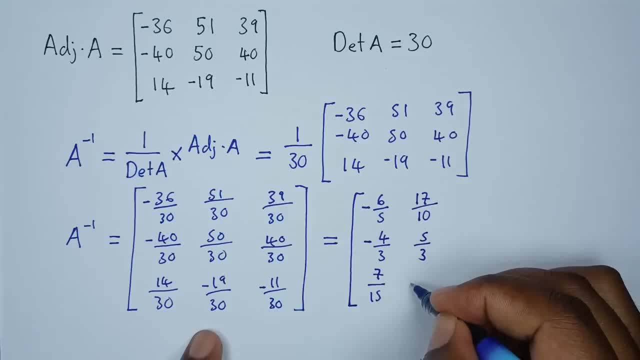 hence we have 5 over 3.. we come here, leave it as it is: 19 over 30.. here we can reduce it by including a 3 into both. so 3 into 39 should be 13 into 30 should be 10.. here we cancel the zeros. 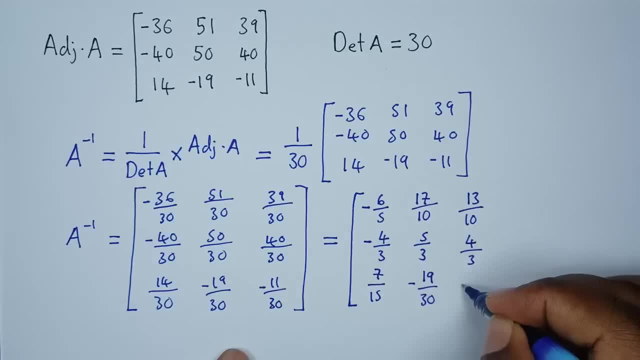 we have 4 over 3 and, lastly, this can remain as it is, which is 11 over 30.. so this is the inverse of that particular matrix a that we had so remember. uh, the first step, let's just quickly go through. the first step is, uh, to find the determinant that is on matrix a, find the determinant, the. 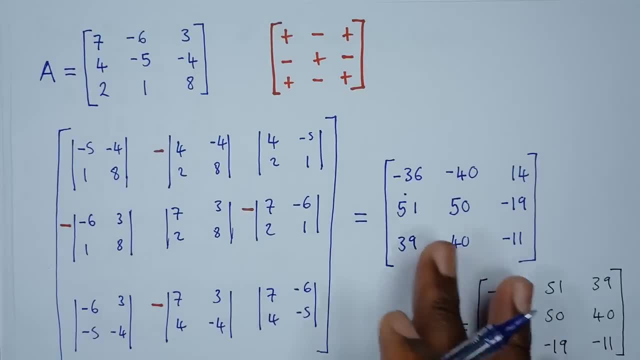 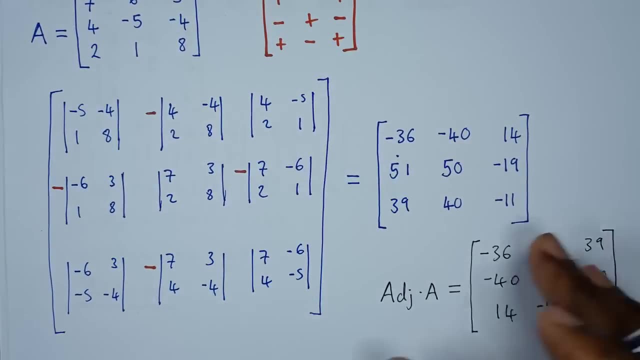 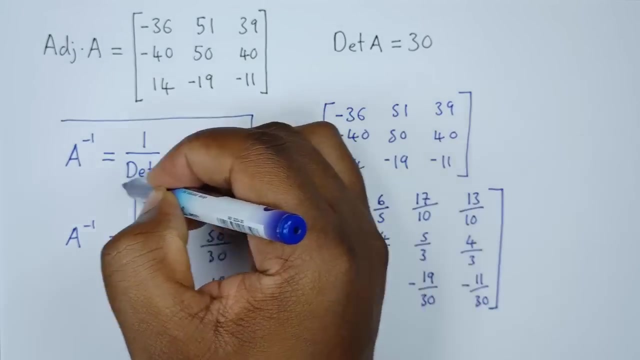 second step, after finding your determinant, is to find the cofactors. after your cofactors, whatever you have here, you transpose. if you transpose this, what you get is your adjoint. then, once you have your adjoint and your determinant, you just come and apply this particular formula that we have here and that gives you the inverse of this matrix. so 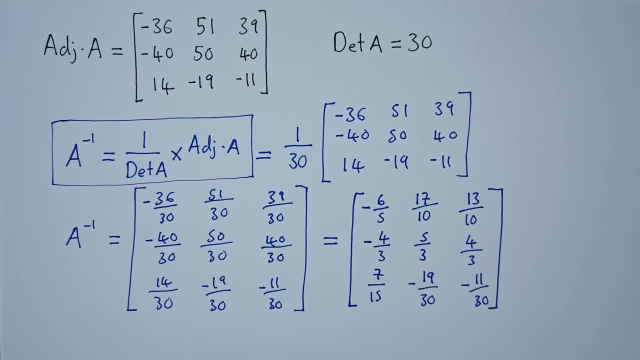 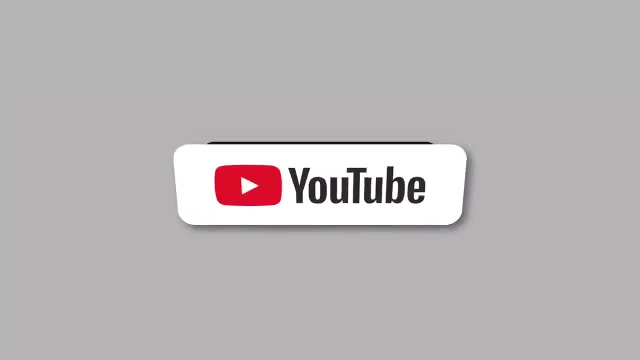 in case you have a question, please feel free to drop it in the comments. thank you very much, you.